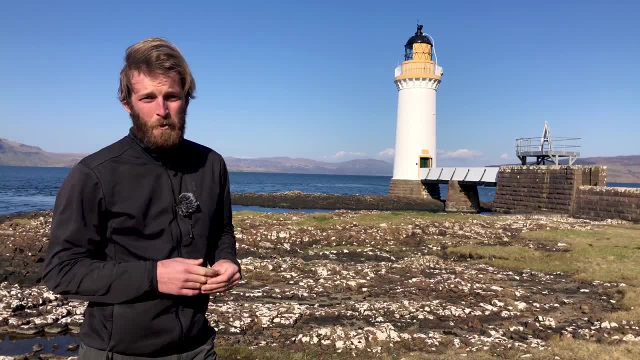 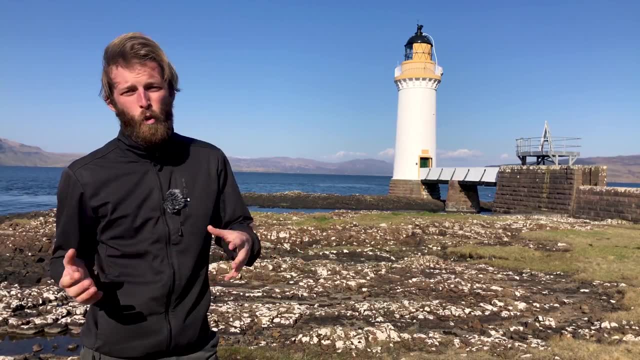 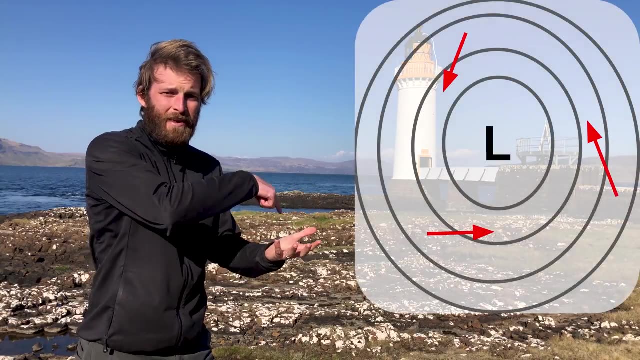 high pressure systems and low pressure systems, but it's not quite so straightforward. The air moves directly from the center of one to the other. What actually happens is, in the northern hemisphere, the wind rotates around a pressure, a low pressure system, in an anti-clockwise direction. 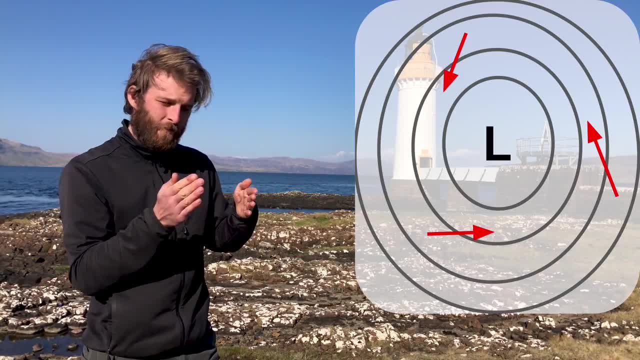 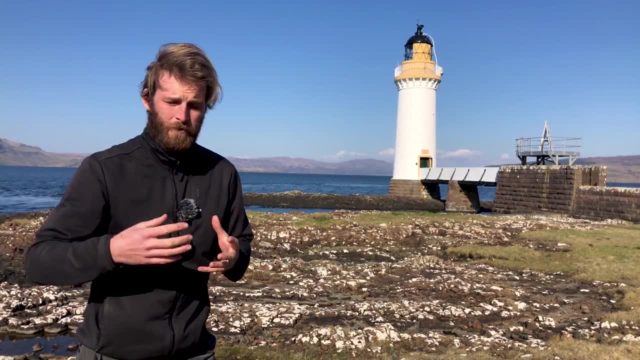 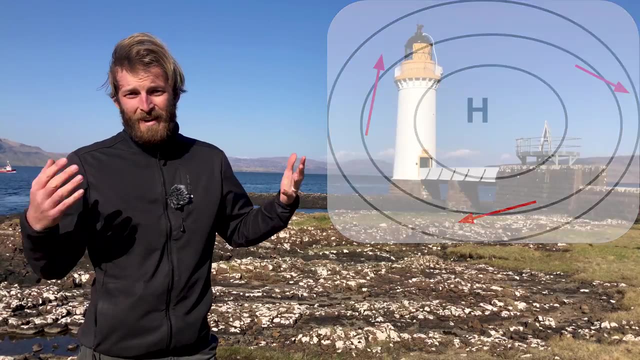 as it is moving in. So it's slightly towards the center, but also around an anti-clockwise High pressure systems. the opposite happens. The wind is blowing out slightly, but also in a direction. Now the bizarre thing is in the southern hemisphere it's the other way around. 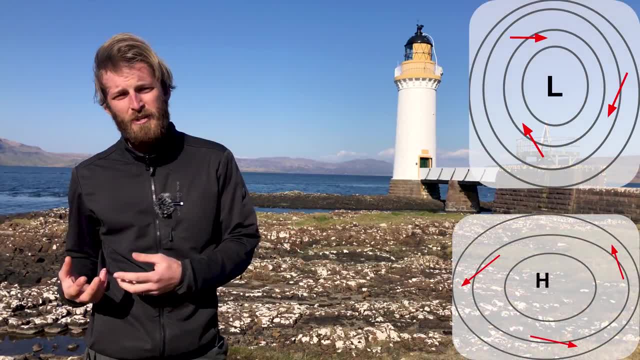 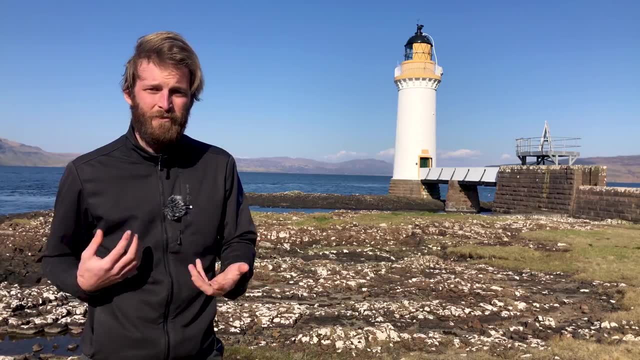 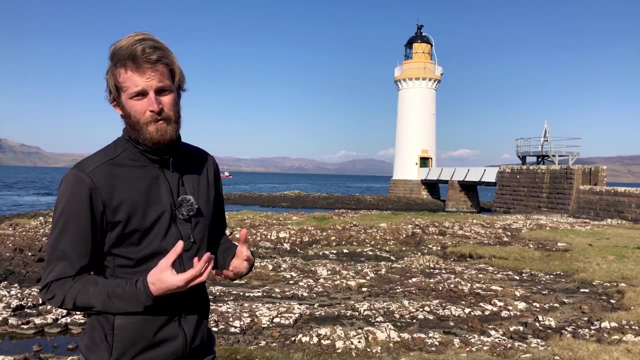 So the low pressure will be clockwise and the high pressure will be anti-clockwise. You're probably wondering why on earth is all this air spinning in different directions? Well, this is actually all due to the earth's rotation and what we call the Coriolis effect. Now I'd love to go. 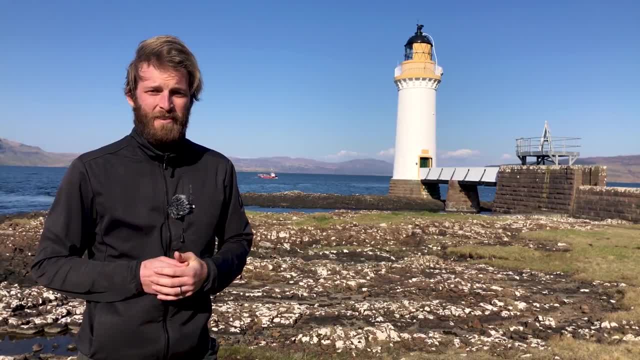 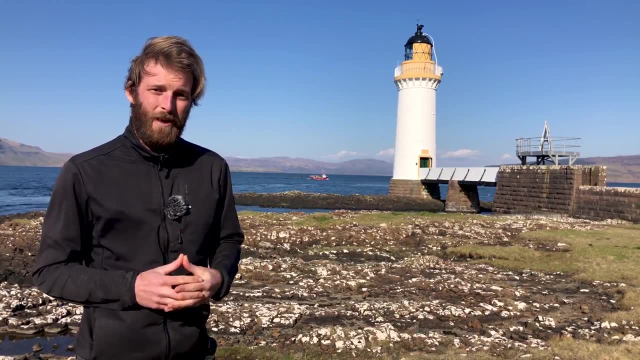 into some real depth about this, but, to be honest, I don't think it's going to be that easy. I don't think it's going to be that easy because that's an entire course in itself and we're not here on a meteorology degree. So that's all I'm going to say for now, and we'll keep moving on. So here we've. 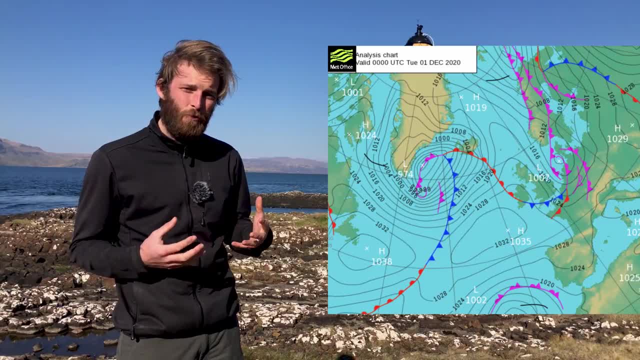 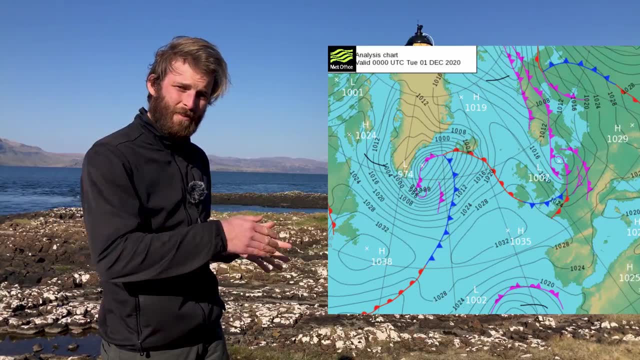 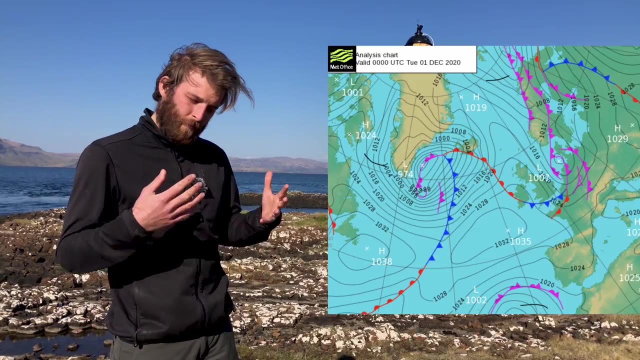 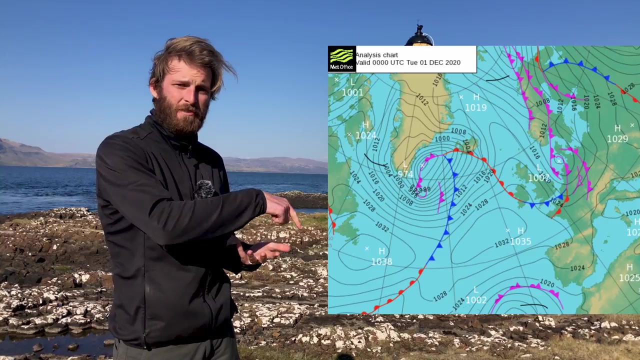 got an example of a synoptic chart. Now this is what meteorologists put together to overlay the pressure systems onto a map of the earth, so we can start to interpret the weather. Now. it looks complicated at first, but it's actually quite simple. All those little black lines all connected in circles around the pressure systems. 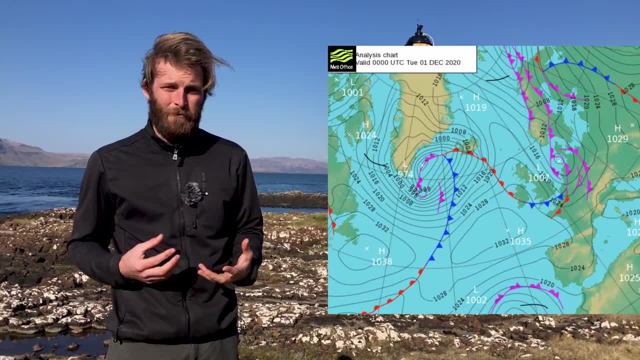 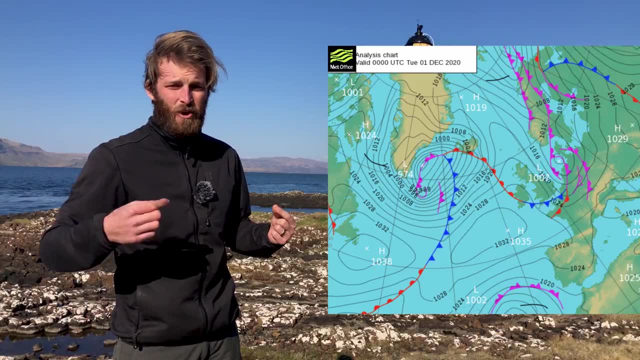 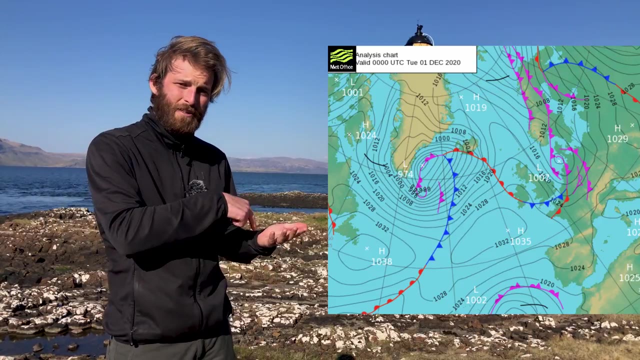 are. those are isobars and they work a lot like depth contours. Depth contours join areas of the same depth. Isobars are connecting areas of the same pressure, So everywhere on that line is the same pressure. The wind will be following those isobars around a low pressure They'll be following. 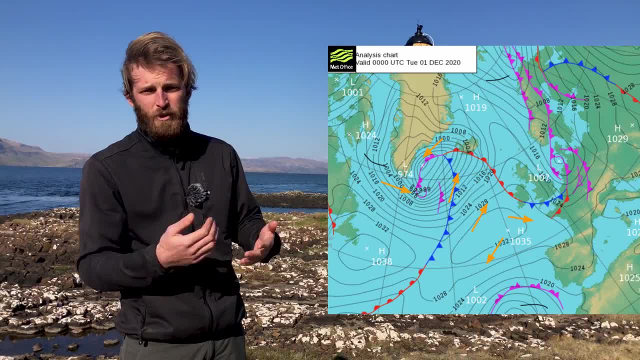 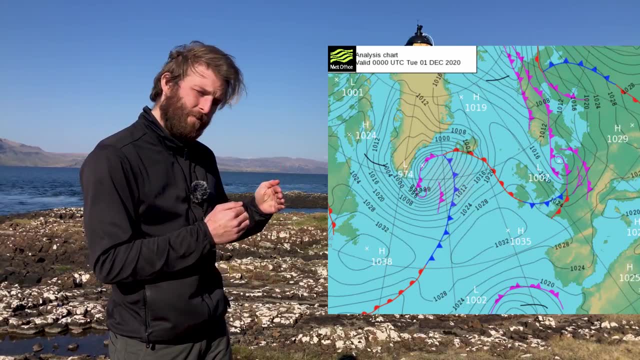 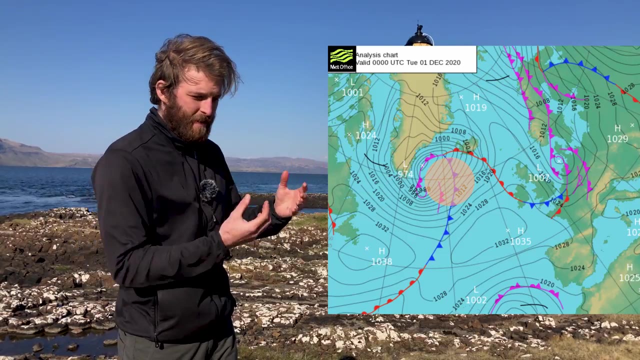 in a slightly clockwise direction and slightly inwards, and the high pressure will be the opposite. Now, a key thing to see here is that the closer those isobars are together, the stronger the gradient from high pressure to low pressure. The steeper the gradient, the stronger the wind. 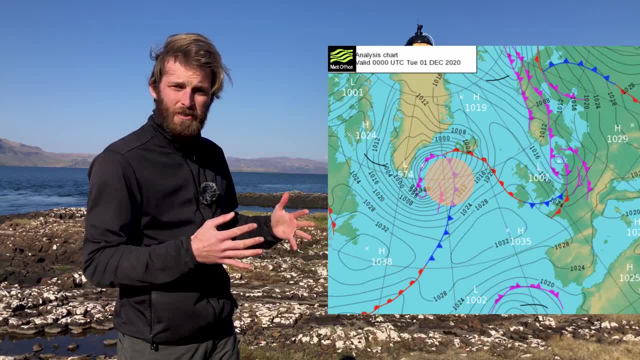 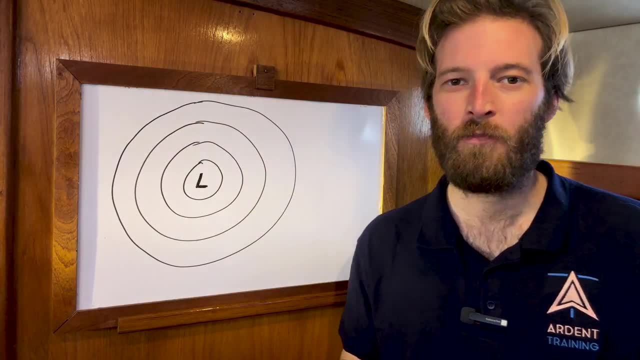 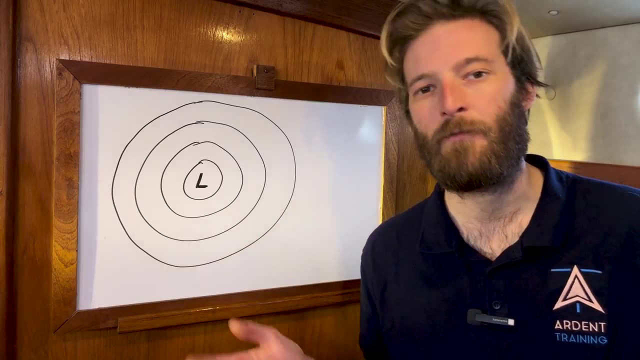 We couldn't stay in the sun all day because this bit is a little bit more complicated and I'm going to need the trusty whiteboard to help with this one. We're going to start looking a little bit more in depth at low pressure systems. just what I've drawn on the board here, So what we already 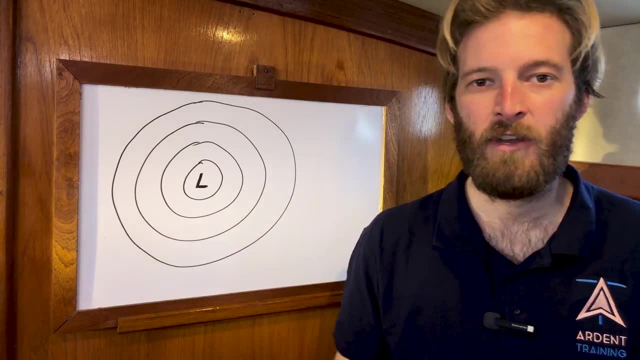 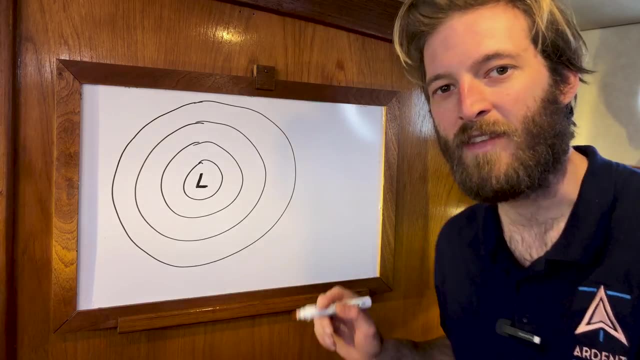 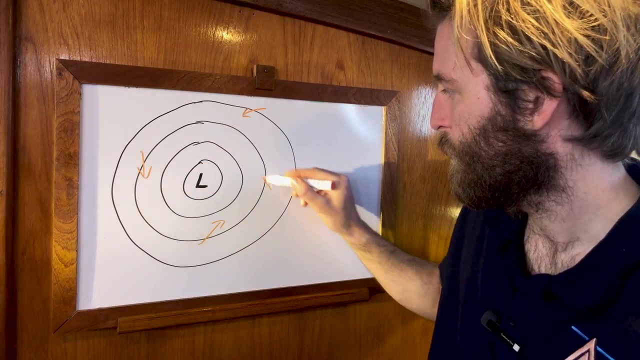 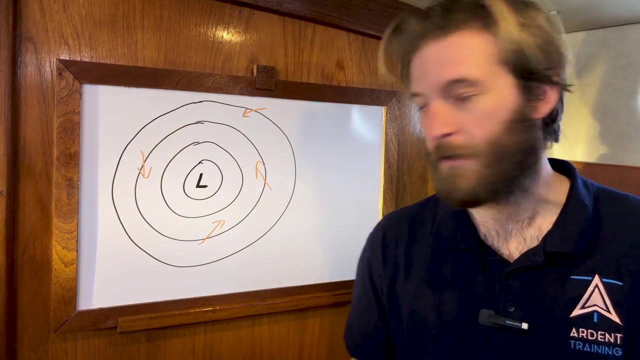 know is that the wind, the air, circulates around a low pressure system in the northern hemisphere in an anti-clockwise direction and slightly in towards the center. There we go. So those orange arrows represent the wind direction, and that should be familiar to you already. Now what we haven't previously discussed is that, as these low pressure systems move across the surface of the earth. they pick up different air masses from different places, some warmer and some colder, And remarkably, warm and cold air does not mix very well at all. The heat does not transfer from one to the other. 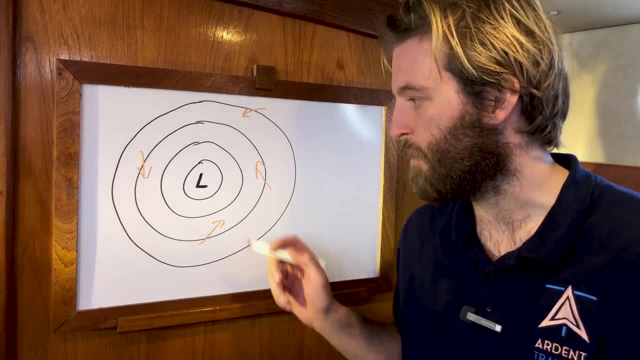 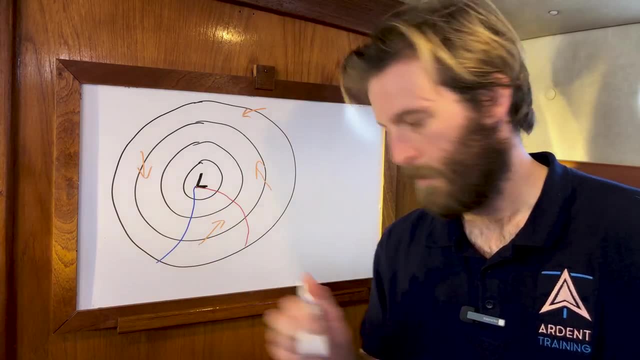 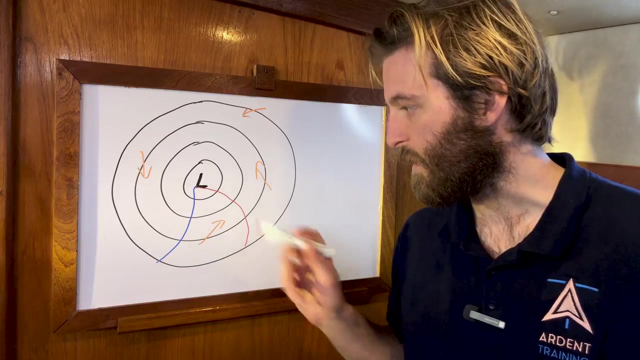 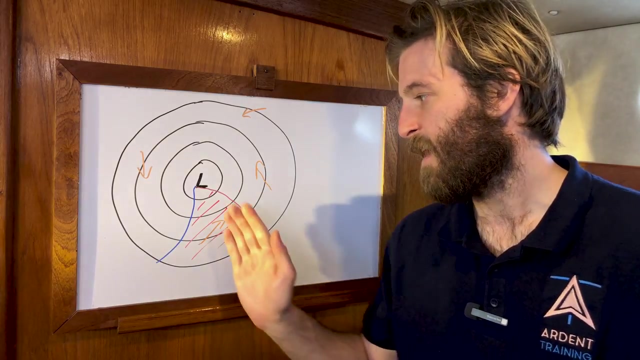 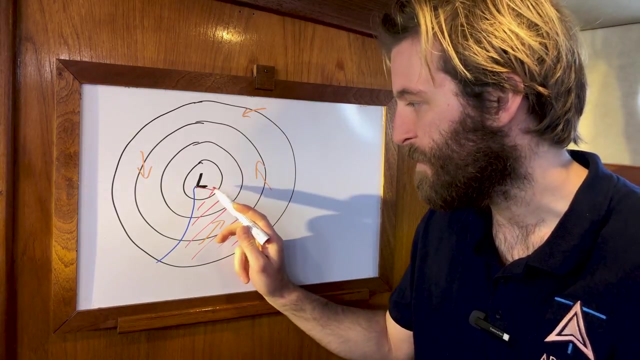 And so you get pockets of warm air and pockets of cold air. So here we have a pocket of warm air circulating around this pressure system and everything in here is warm. Now, at the front, as at the front of this warm sector, we're going to call it the warm front, And this is labeled. 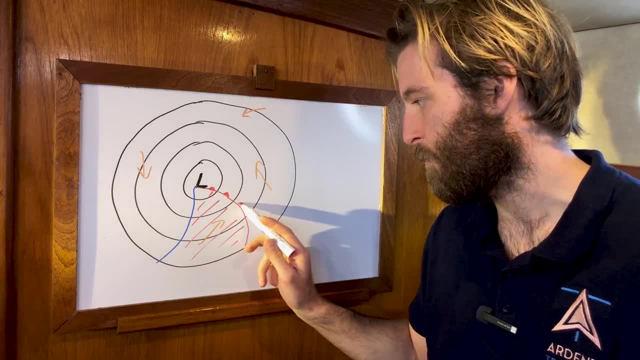 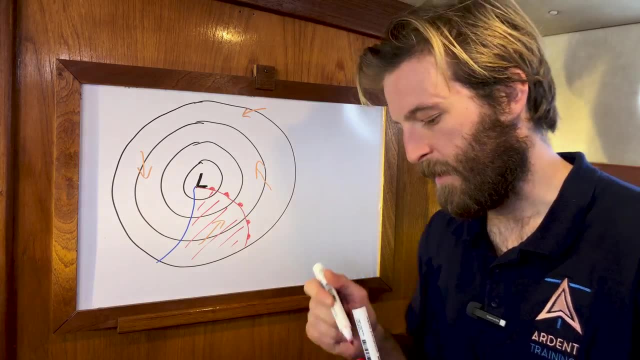 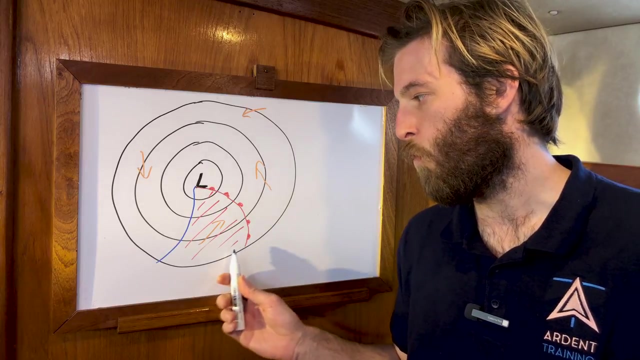 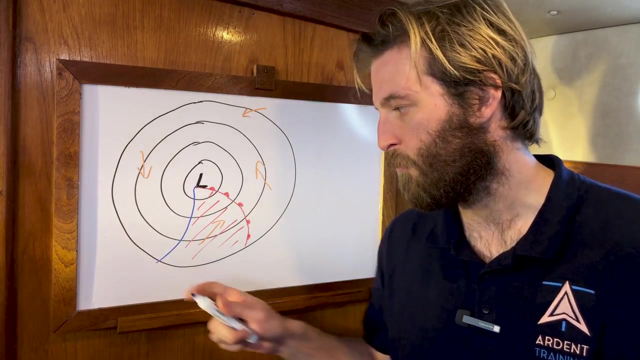 with little red semicircles along the leading edge of the warm front. This just indicates it is a warm front and the direction it is moving in. As that passes over we enter the warm sector and as the warm pocket of air passes, we'll get a cold front. 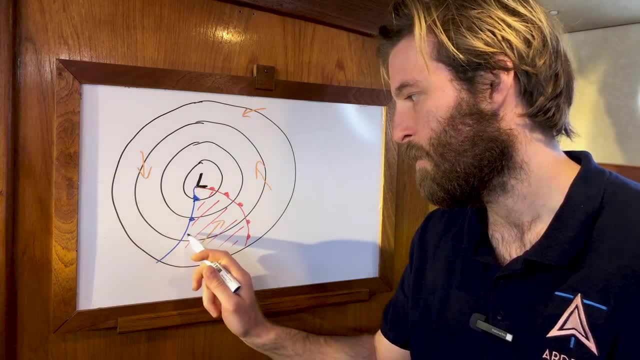 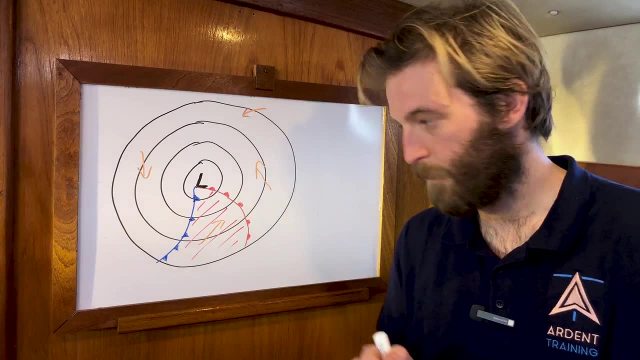 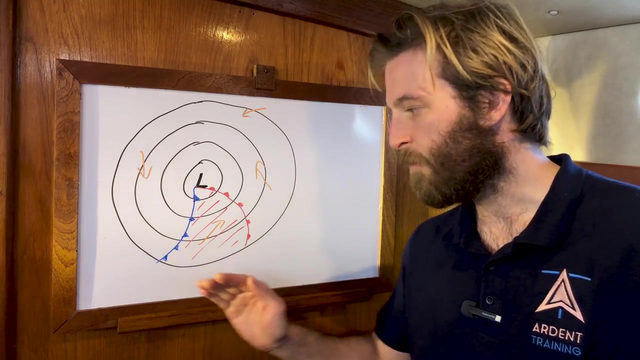 which is labeled on our synoptic charts by a blue line with little blue triangles. So this is how it would look on a synoptic chart. The reason this is important is because, as this warm front passes over, as we're in the warm sector, and then the cold front, 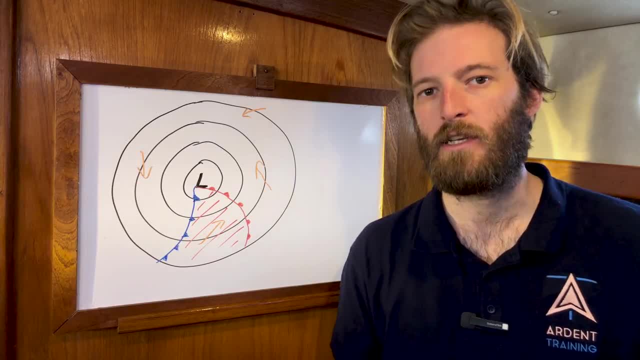 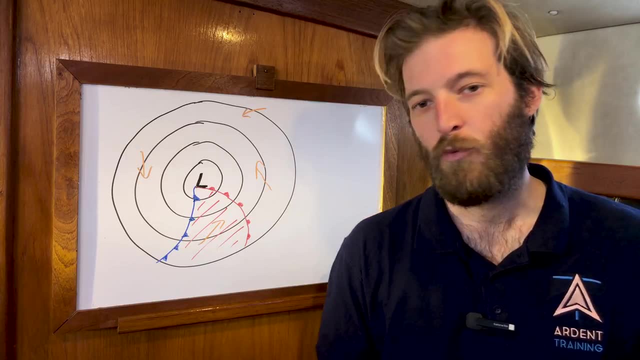 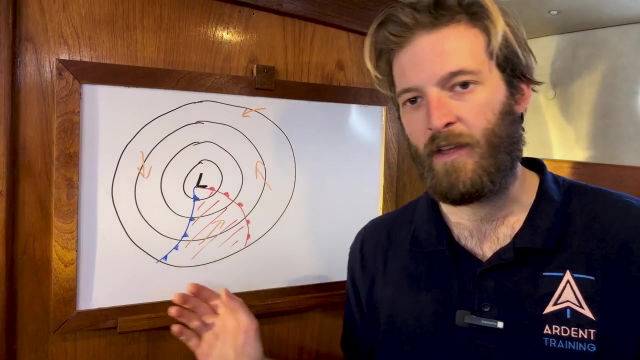 this brings quite a lot of rapid changes to our weather. The winds will change direction, it will increase or decrease in strength, and we might get rain or poor visibility. So it's important to understand how this works so that we can predict what weather. 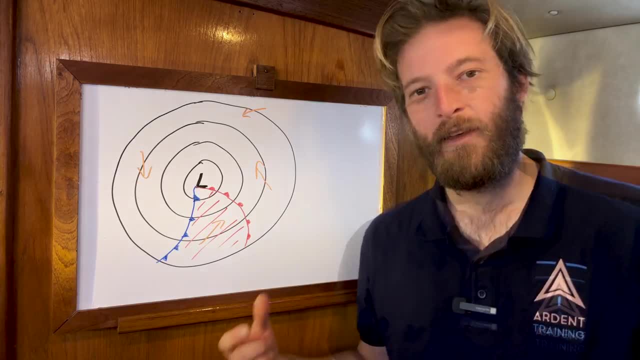 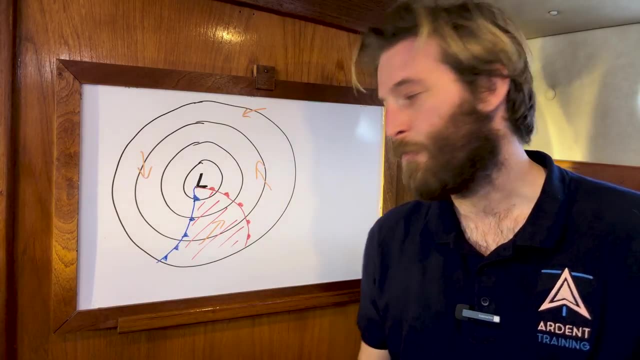 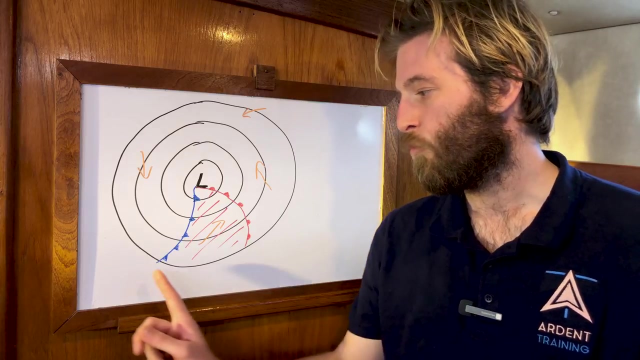 is going to be approaching us. One reason why this warm sector is so small relative to the high and relative to the whole low pressure system is because the cold front actually travels a lot faster than the warm front, and so it is always catching up with the warm front Eventually. 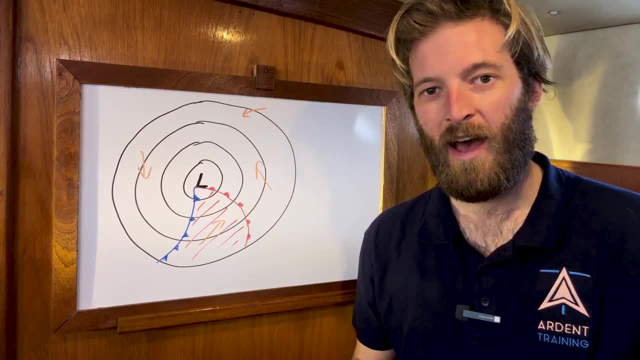 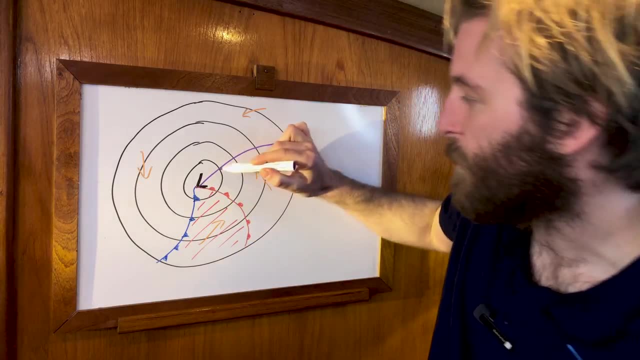 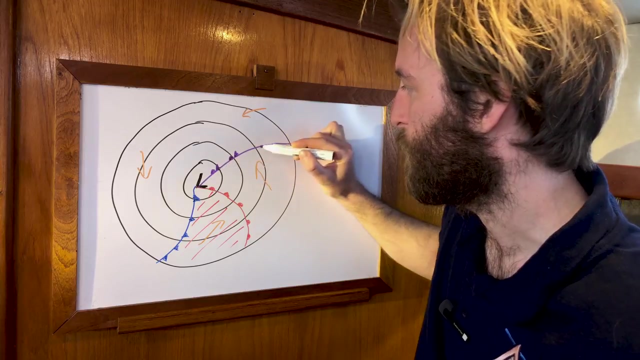 it will catch up and overtake the warm front and, in place of a cold and a warm front, we will instead have an occluded front. An occluded front, if it was coloured, would be purple, and it has semicircles and triangles indicating that it is an occluded front and the direction it is. 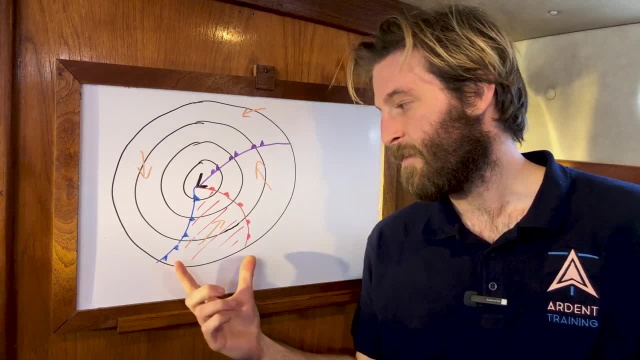 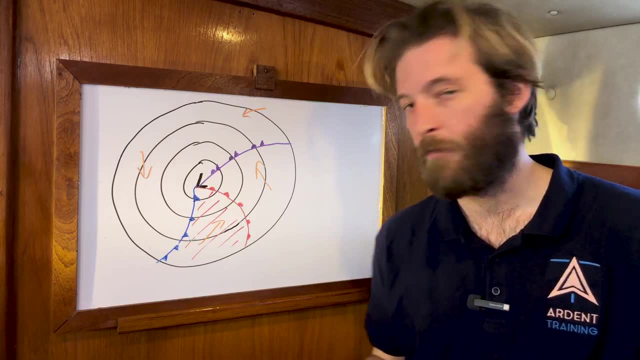 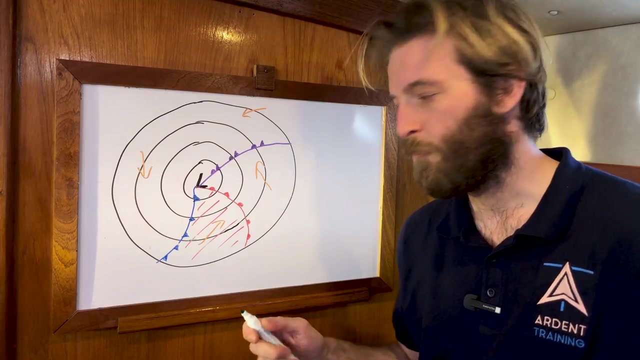 travelling in. I mentioned that, as this warm sector passes over us and the front, we're going to see some rapid and sometimes quite drastic changes in the weather, and that's what we really need to focus on. So, to explain this better, what we're going to do is we're going to take a cross. 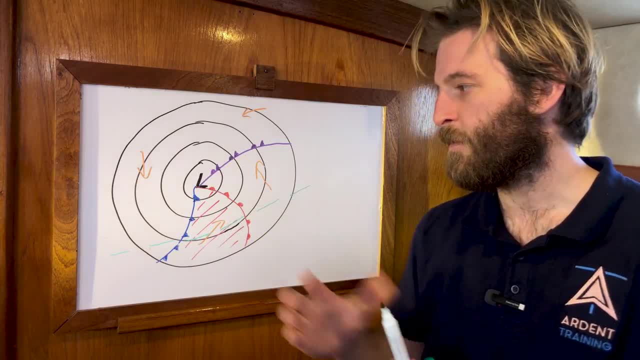 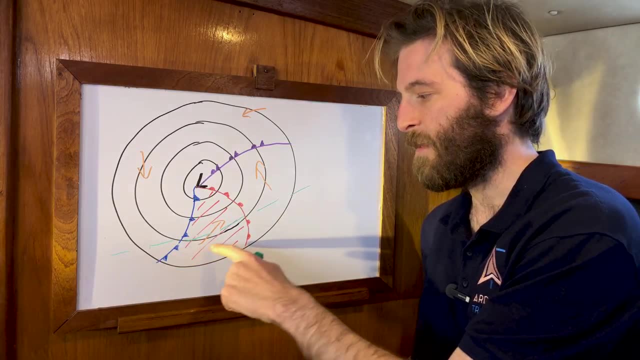 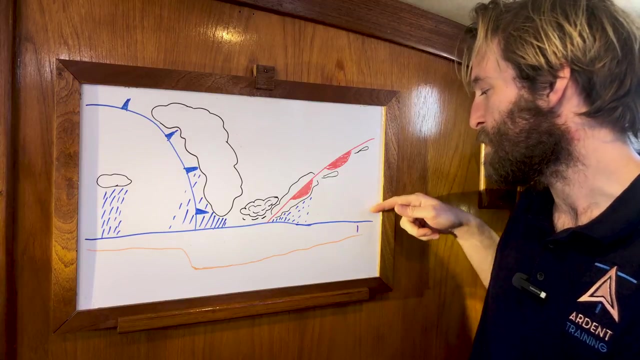 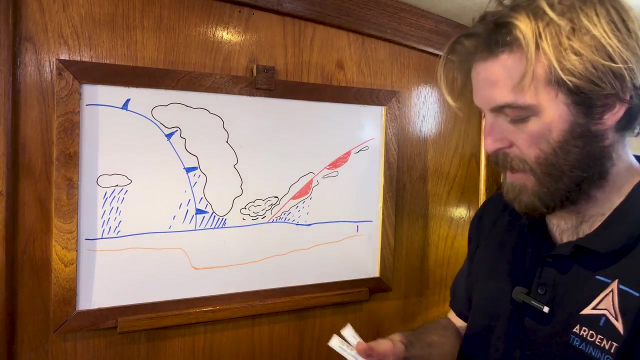 section of this pressure system. at the moment this is a top down view, but we're going to change it to a horizontal view and see what happens as these fronts pass over us. Okay, let's start here, point number one: we are just underneath the start of the warm front, so this is the warm front here and in the middle here. 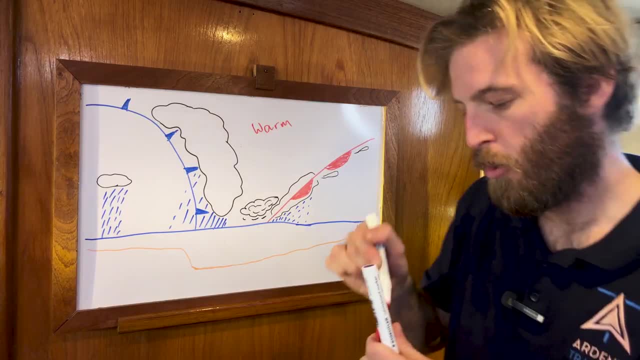 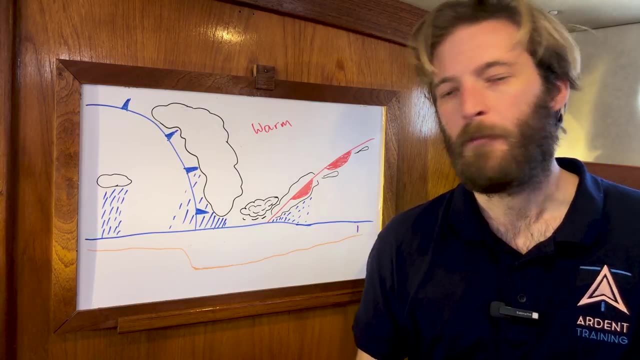 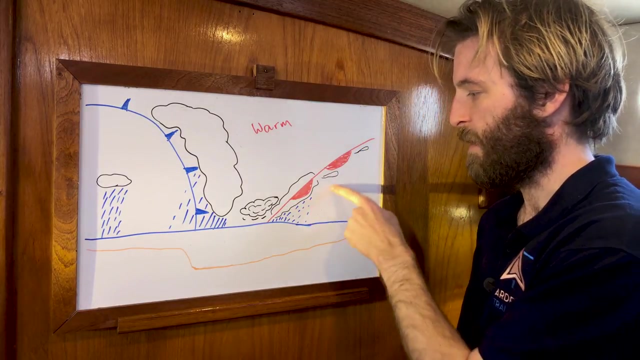 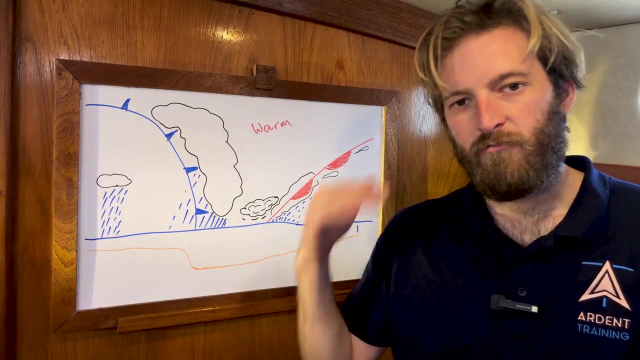 this is the warm sector, full of warm, buoyant, low pressure and moist air. Because it is warm, it is less dense, it is rising above the cold air that we are currently in, and so it's staying relatively high here. it's going to start affecting the weather really far above us, at the where it meets the cold air. we're going to start 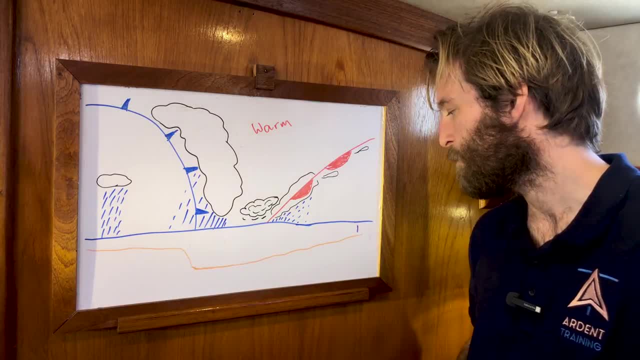 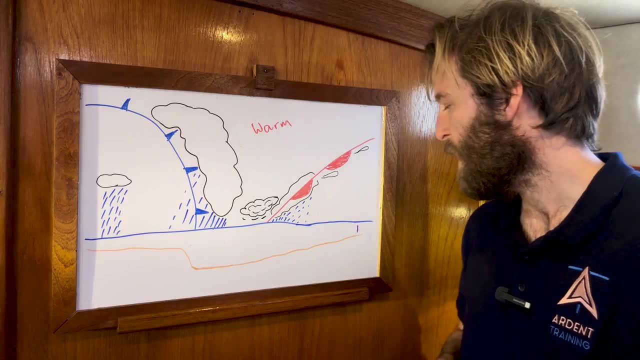 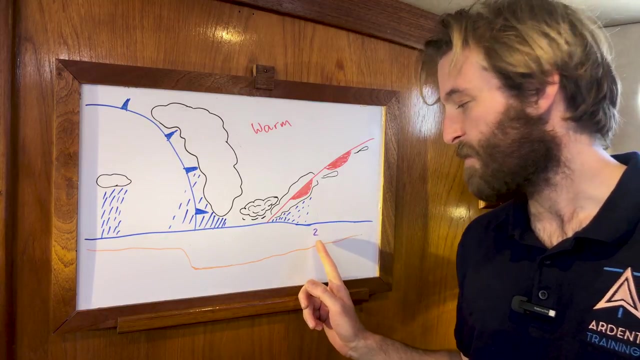 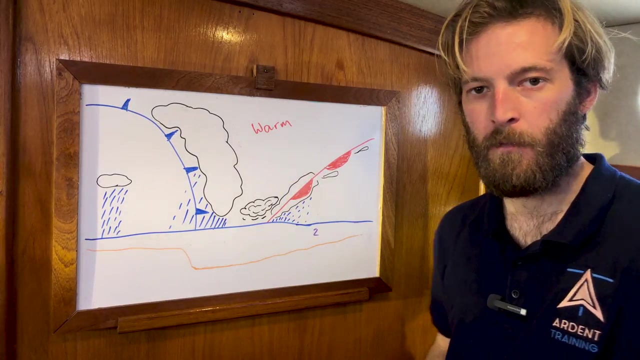 getting some very high clouds. really high up We can also expect to see the bright, medium and low wind, And here we are looking at the Arctic Ocean. We have some very warm air there. We can see the mild air as the clouds are fastening and getting more thicker there. 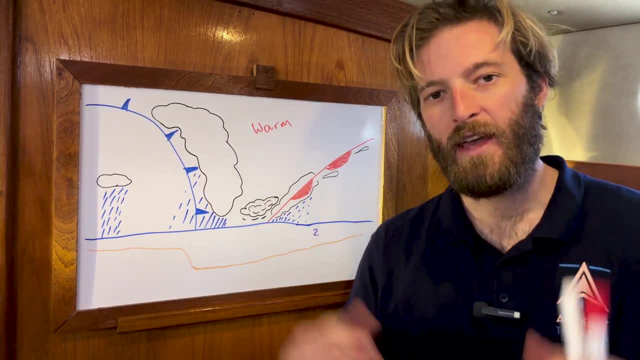 Our speedometer starts to steadily fall, and the wind may just start to veer and increase a little. Moving on to our second position in our passage of fronts here, the warm air is getting much closer. now. there's less of a cold layer between us and the warm, and so the clouds are also getting lower down. as they're getting lower, they're getting thicker and they are starting to fall. 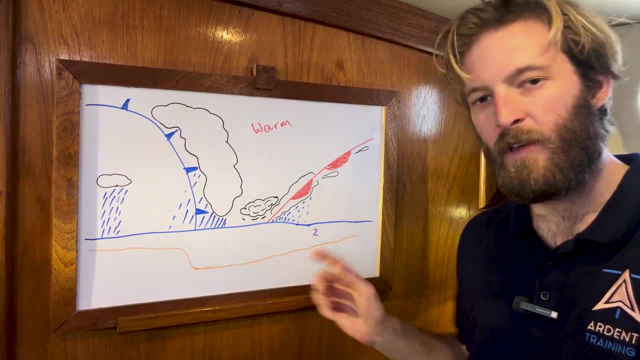 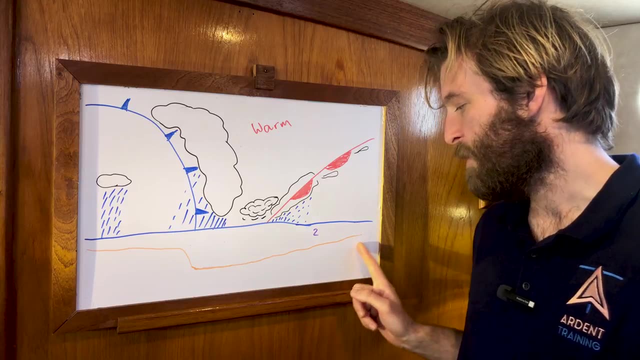 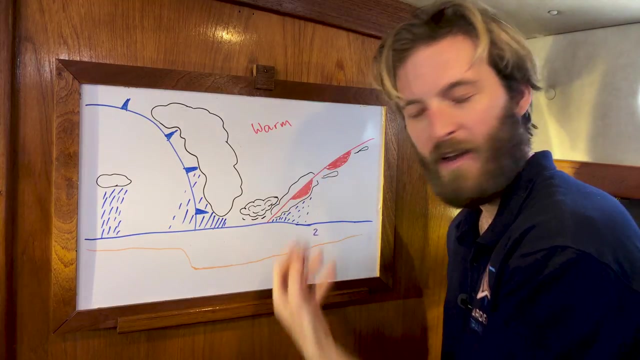 rain on us. We might have had some very light drizzle before, but it's now going to get much more steady and heavy. The barometer is going to continue to fall. Remember: this warm, light air is going to be have less weight to it. It's going to be less pressure on us. 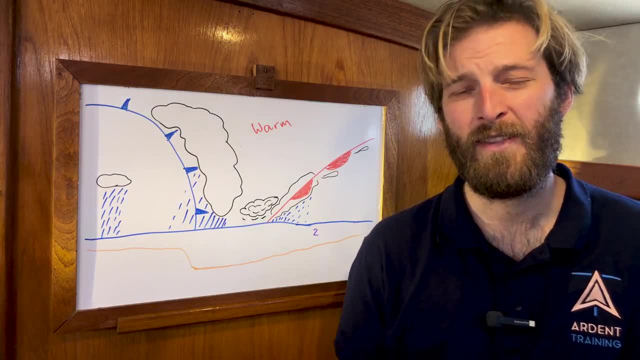 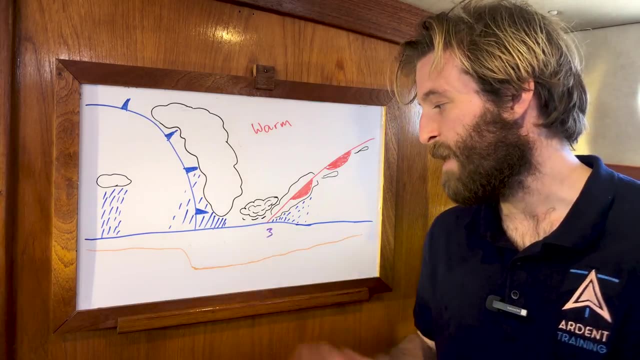 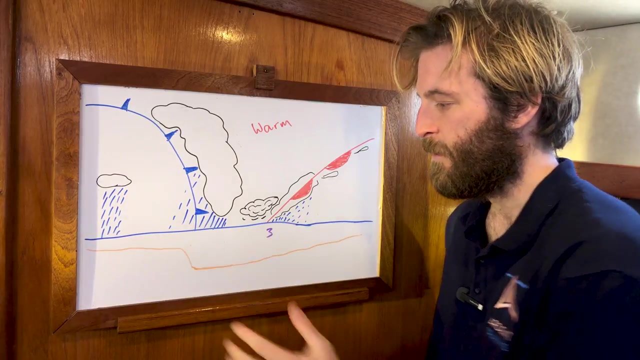 So our pressure will steadily continue to fall and the wind will carry on veering and increasing slightly. Here we are now at point three, and the warm sector has hit us. It has all the cold air has blown away and we are now entering a wide area of warm air. Now, this warm. 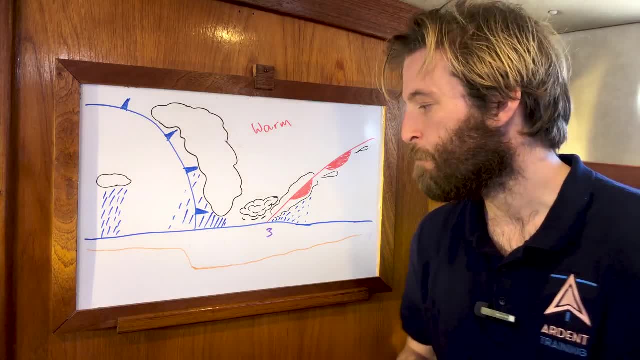 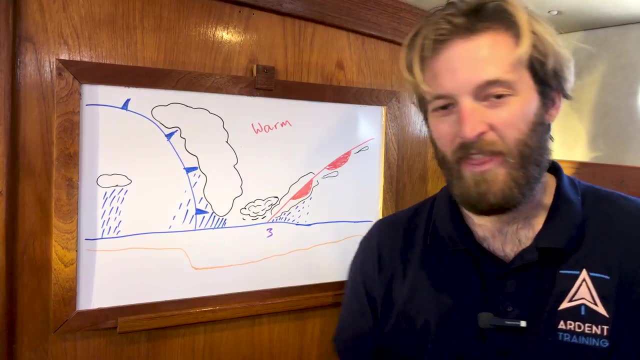 air is going to be moist. It's going to contain a lot more moisture, And what that's going to do is bring some really low cloud down to us- low cloud and drizzle, And this makes for really poor visibility. So that's an important one. 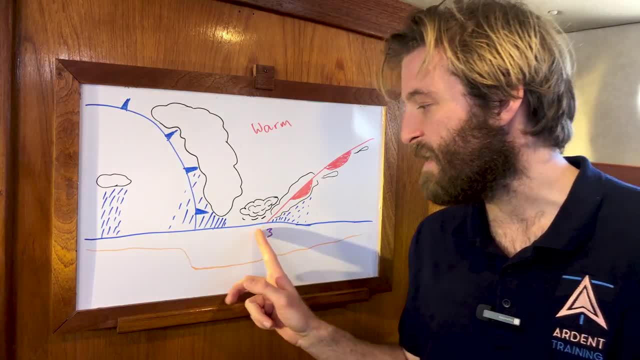 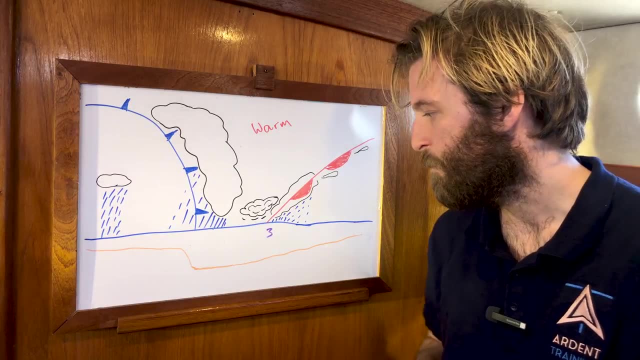 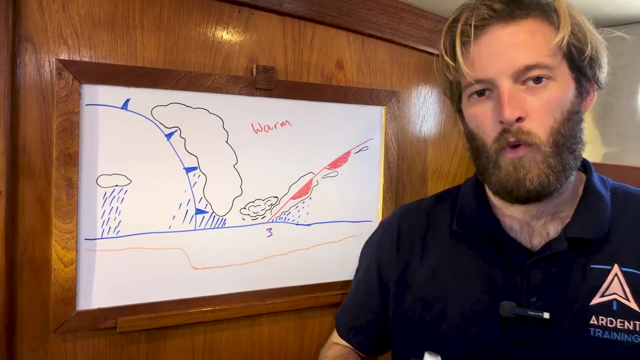 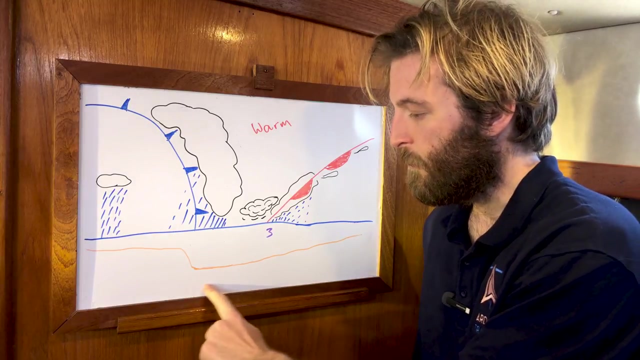 If we can see this warm sector coming up, that's not a great time to be undertaking some tough pilotage. Now, though, we are entering a much more stable part of air, where we are no longer changing from one sector to another, And so the barometer has steadied off. It has gone down a 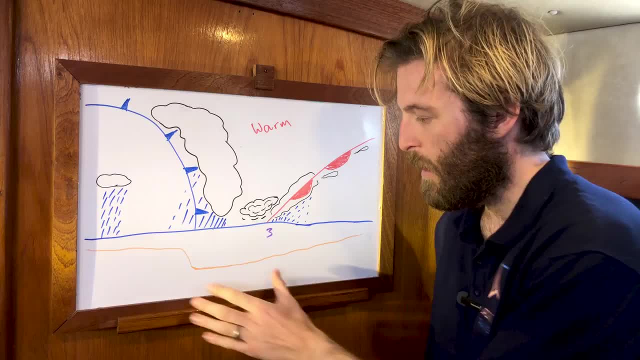 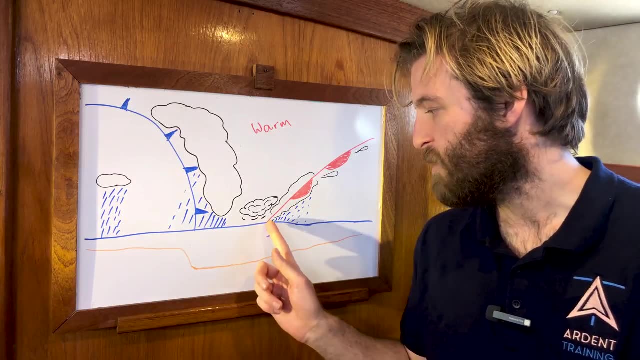 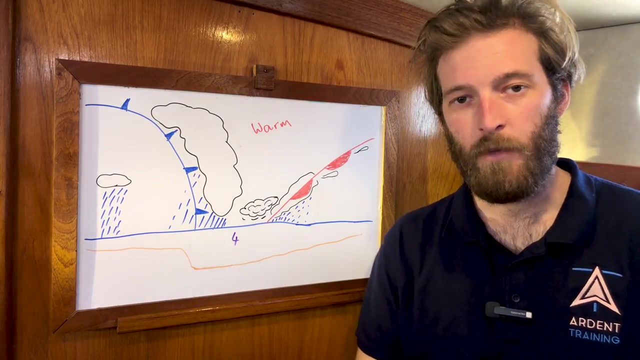 long way. Remember, the warm air is more buoyant, There's less pressure, but it will not be changing for a while. The barometer is steady. The wind may veer a little more, just as this warm front passes over us. Okay, position number four in our passages of fronts, And we are nice and stable in the warm. 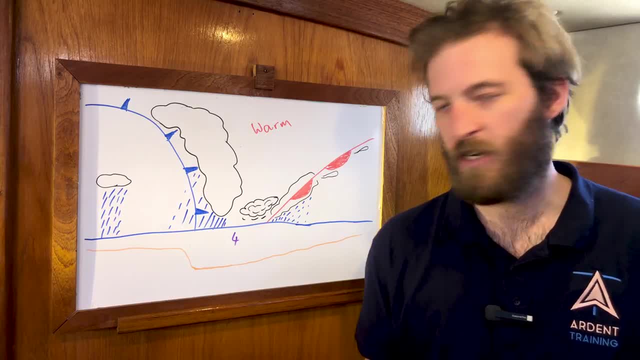 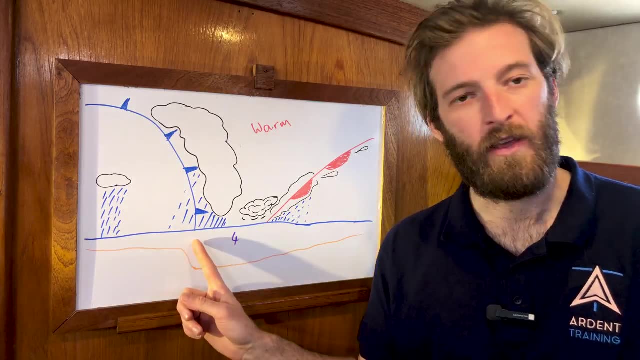 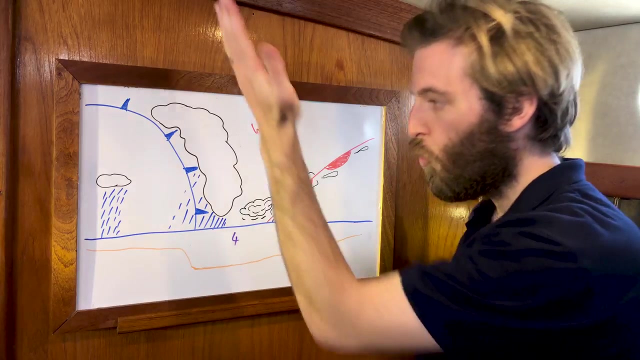 sector. The barometer hasn't changed for a little while and it's not going to change for a little while longer. The wind is steady. However, this cold front is now fast approaching. This cold front is coming in and cutting underneath the warm air and pushing the 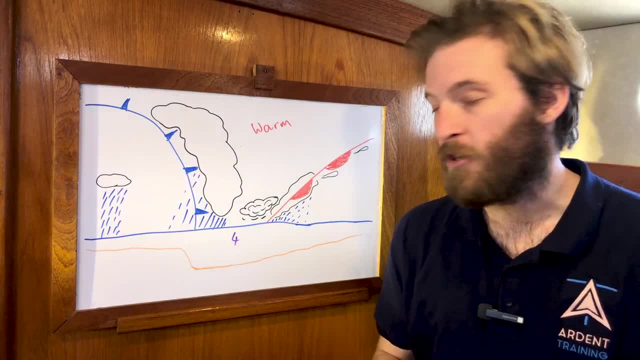 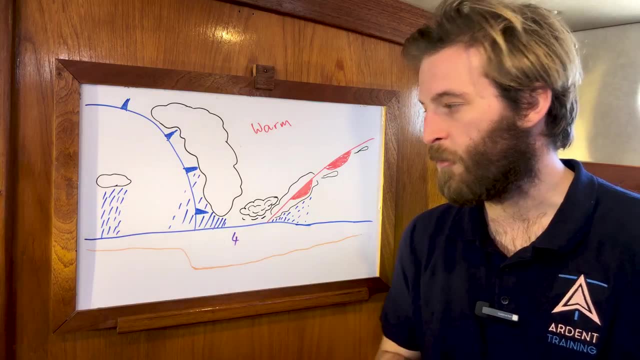 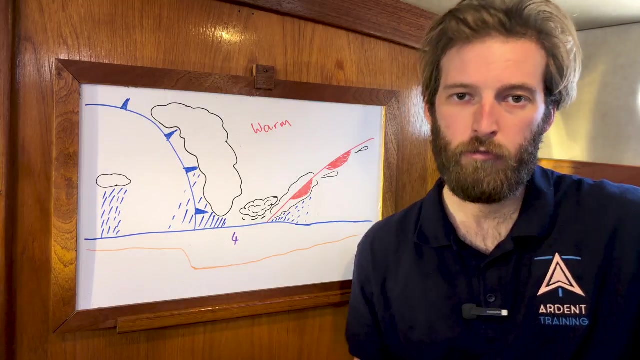 warm air up. What this is going to do is create a lot of vertical movement in air. This air is going to be rushing up and down. It's going to be turbulent as this cold front approaches. So now we're here, we're going to have to start looking forward and looking out for high towering clouds. 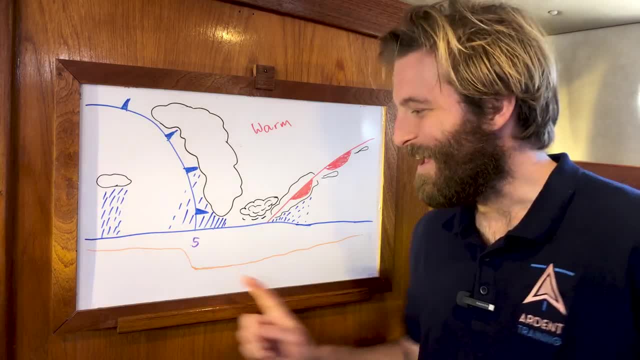 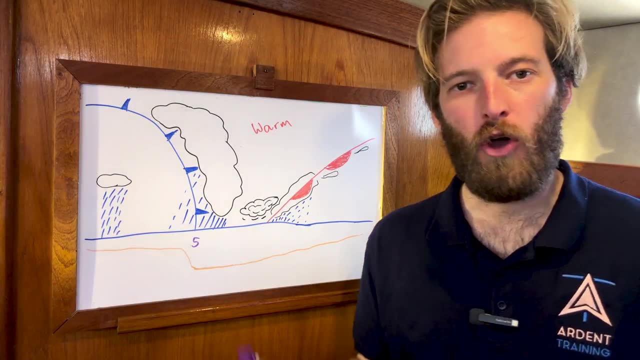 which might bring thunder and heavy rain. Here we are at point number five And the cold front has hit us. We are now moving into this big sector of cold air. cold air's, remember, is denser, It's denser, it's heavier, It's going to be. 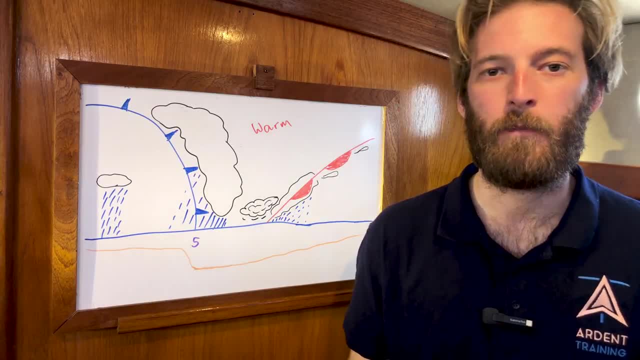 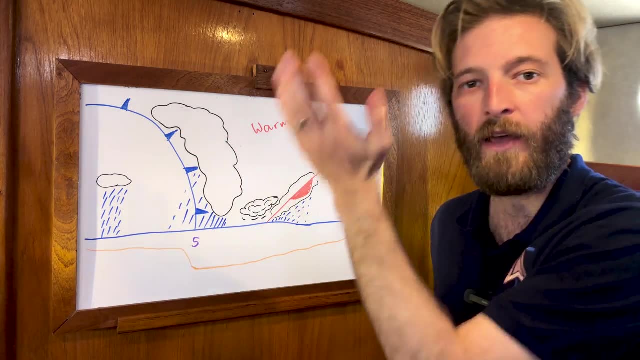 putting on pressure, and so the barometer is going to shoot up under the weight of all this new cold air above us. It's also pushing this warm, moist air up high, further away up into the atmosphere. So the clouds are going to get much higher up, but this vertical movement of the air estar. up, much higher up, But this vertical movement of air at ża nag-kak-j Querartater, Efrat and it is pushing this warm air away further up into the atmosphere. So the clouds are going to get much higher up, But this vertical movement of the air that's very про-sereum. 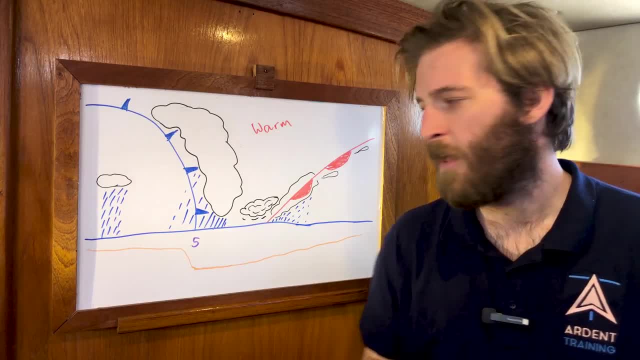 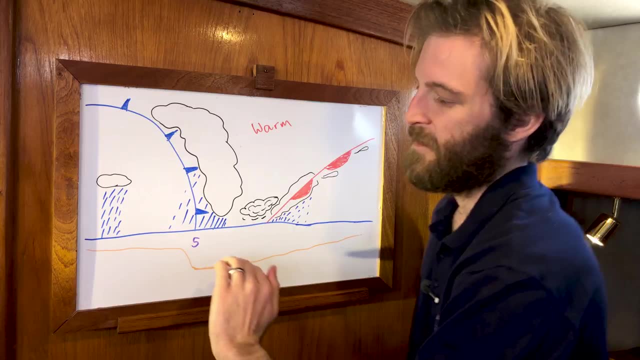 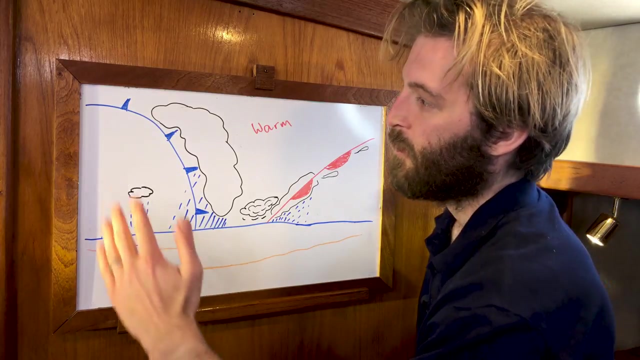 movement of the air could cause some fierce squalls. We can expect to see the wind veer again here. after a steady period where it didn't change, It's now going to veer and we're going to have to look out for these squalls, high clouds and rain. The cold front is pushing away the last of the 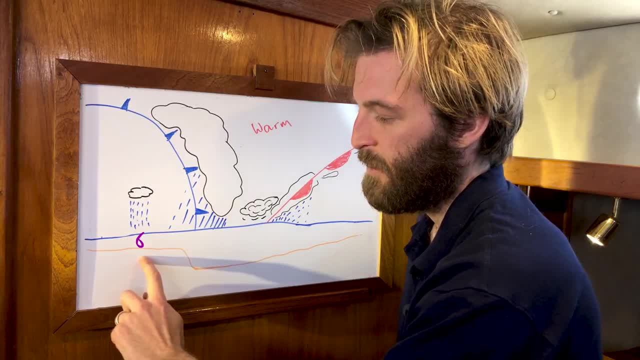 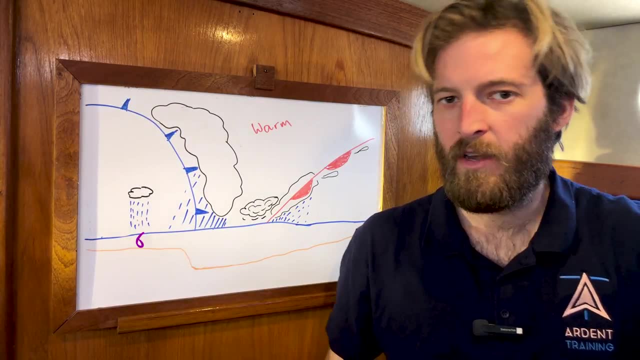 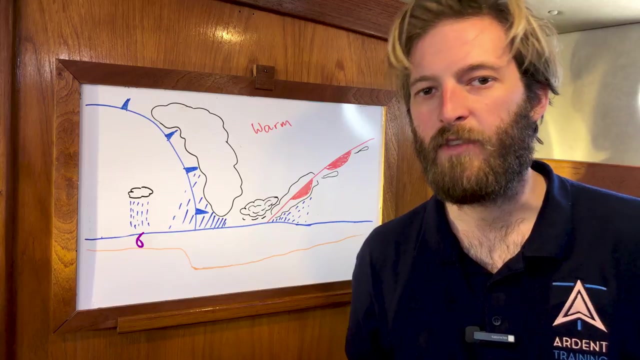 warm air. The barometer is going to continue to rise, but very steadily. now There's not much warm air left to get rid of. The clouds, if there are any, are going to be super high up, and this, this cold air, is going to have much less moisture. It's going to be much clearer. Visibility is going. 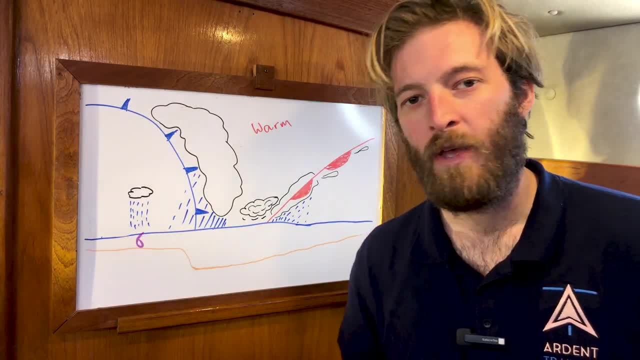 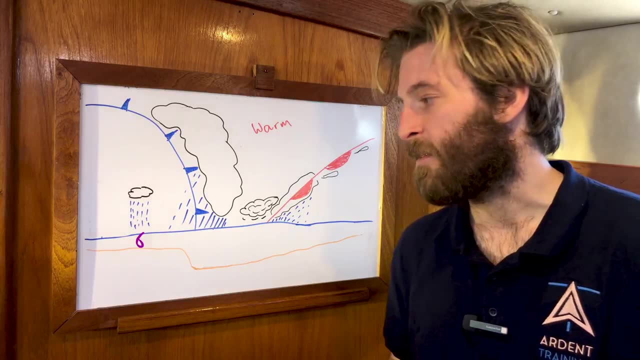 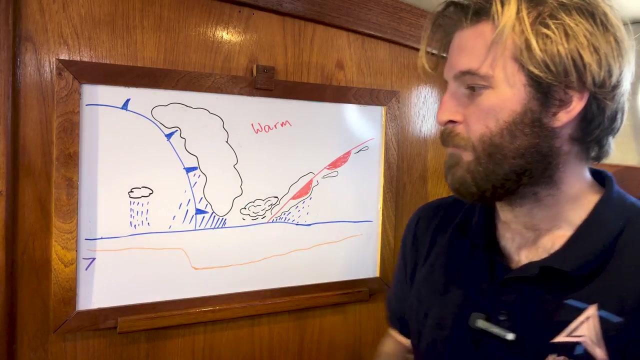 to be really good. However, we might still get some lingering squalls, with rain underneath them and fierce gusts. The wind direction, however, will remain steady, at least Position number seven here. now We're almost out in the clear. We are very much in the cold section. 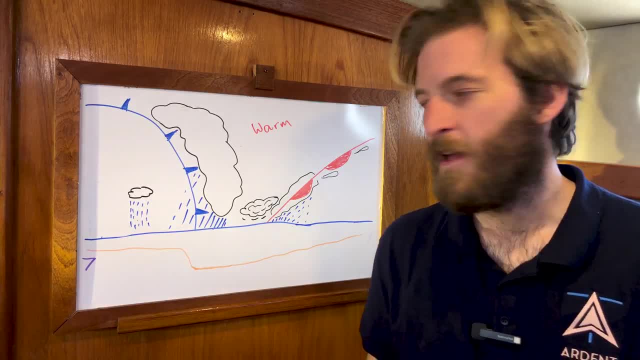 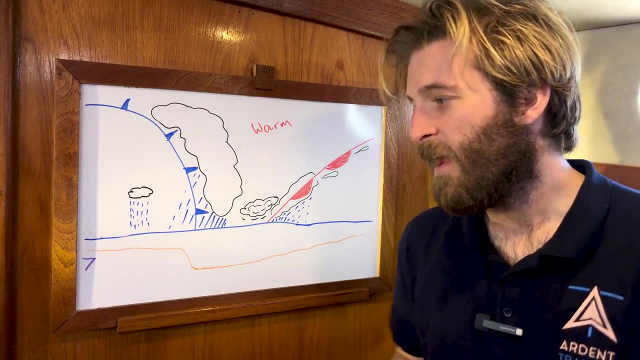 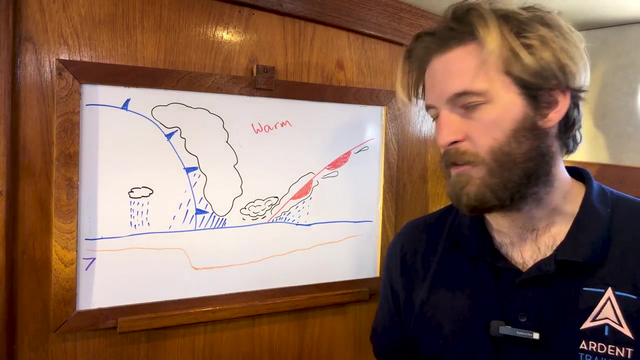 We're going to continue to clear and we're going to have good visibility. The barometer will steadily rise a little bit further and we're going to get much less rain or anything like that. It's much clearer. However, we're still going to get some strong gusts and strong winds that we associate. 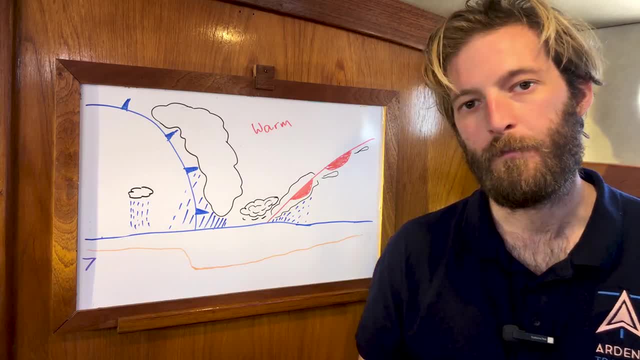 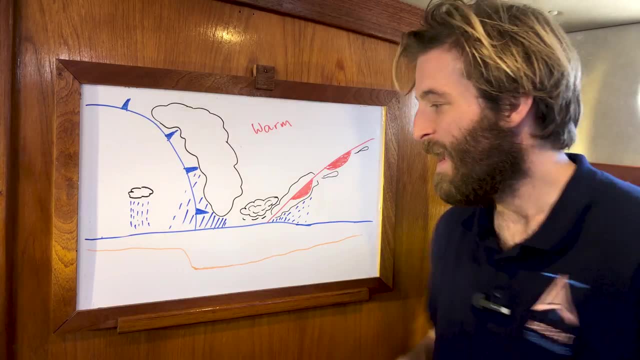 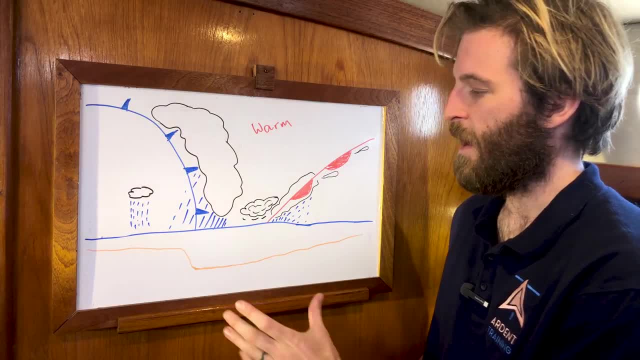 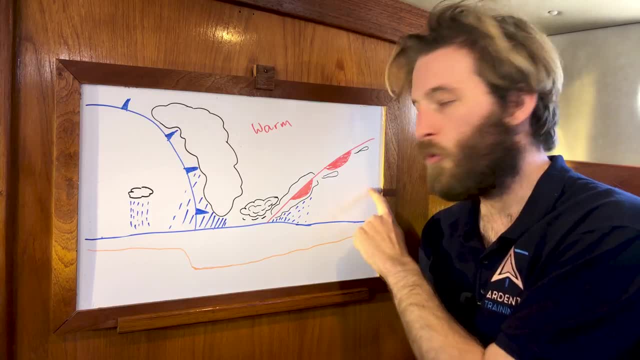 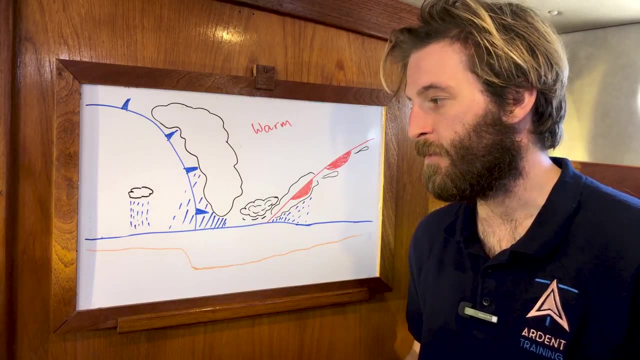 can have a big impact on our day out, And if you can spot the early signs, then you can predict what's going to happen: when it's going to rain, when there's going to be poor visibility, when it's going to get better again. Good news, High Pressure systems are much. 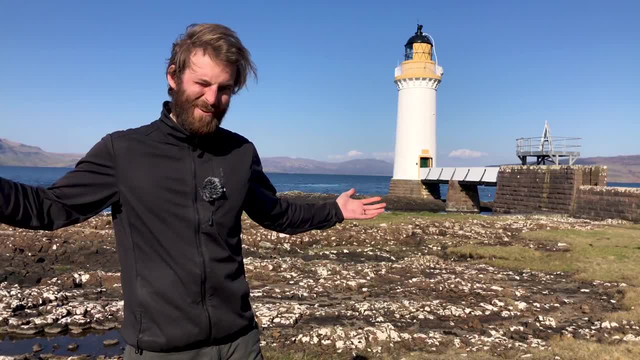 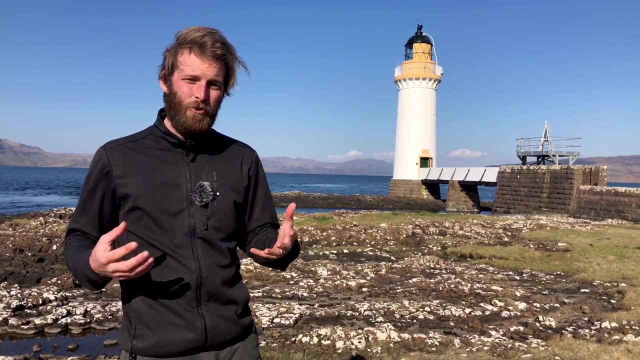 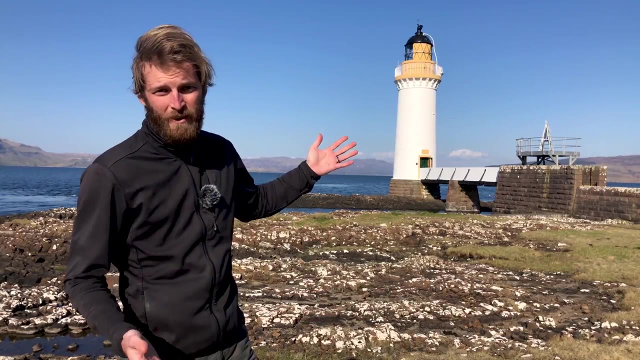 easier to explain, So I've put the whiteboard back away and come back out into the sunshine. Even good news, then, if these high pressure systems are not only easy to explain, they're also very pleasant pressure systems to be in. they create very pleasant weather, just like today. we are sat in a big, stonking high.